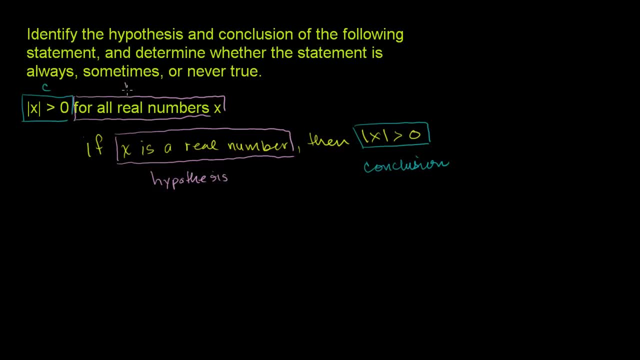 It's a little, a bit easier to identify when you see it written like this: This is the hypothesis. Now, I don't you this. you get confused with the idea of a scientific hypothesis, which is related but a little bit different. A scientific hypothesis is an explanation for some phenomena that 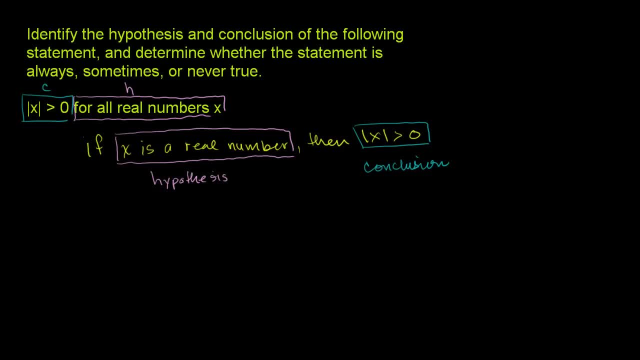 can be tested. So a scientific hypothesis might be something like saying: Blueberries- which I'm writing in blue intentionally- blueberries help reduce the risk of cancer. This, right here, is a scientific hypothesis. You could then go feed a bunch of people- blueberries for a. 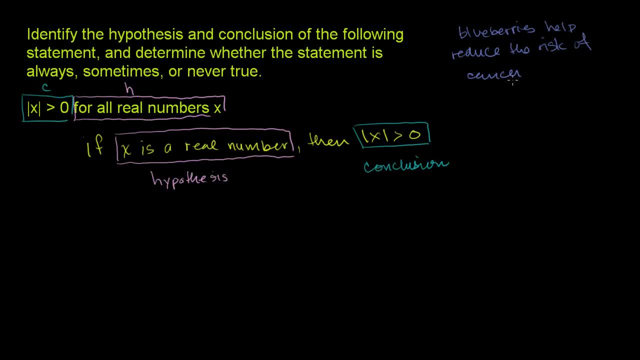 long period of time and see if they have a less likelihood of developing cancer than people who never got blueberries. and everything else is equal, And so it would be testable. You could see if it's true And the conclusion would be whether this is true or not. 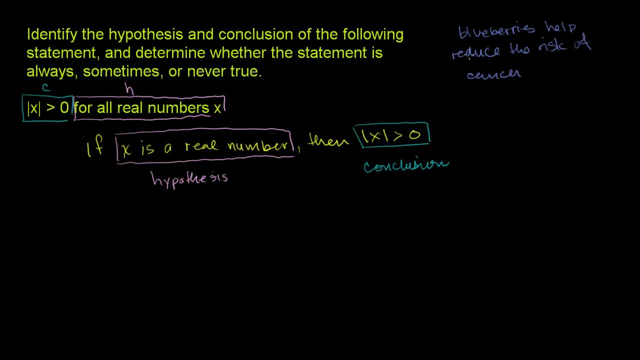 But this is in the scientific hypothesis world, not to be confused with the notion of hypothesis we're using right now, And I don't want to confuse you too much, so I'm just going to leave this on the side here. But when you're in Algebra 1, and especially these are: 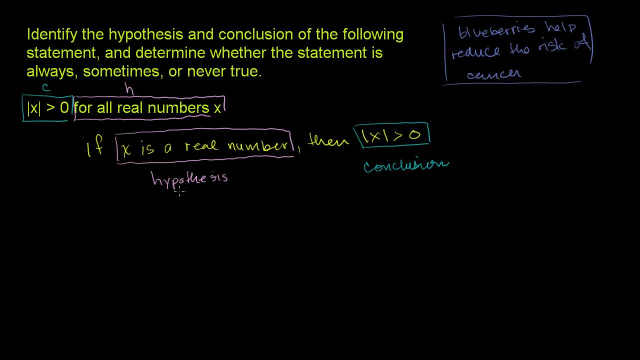 according to the California standards. a hypothesis in this context is the antecedent of this proposition or it's the if part of this proposition? Now, the more interesting question is whether it is true. I mean, we can sit and label statements all day, but that's. 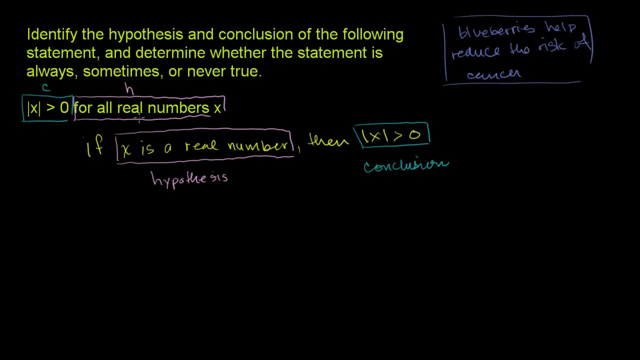 not interesting. The more fundamental thing is: is this a true statement? Is it true that if x is a real number, then the absolute value of x is greater than 0?? Well, the one number that pops out of my mind that disproves. 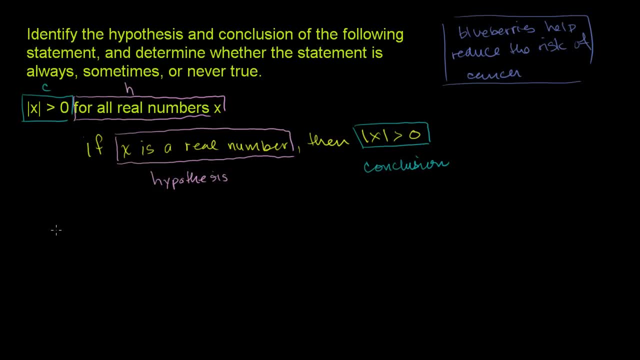 this is if x is 0.. 0 is a real number, 0 is a real number, That's true, But- and I'll write, but in caps- but the absolute value of 0 is equal to 0. It's not greater. 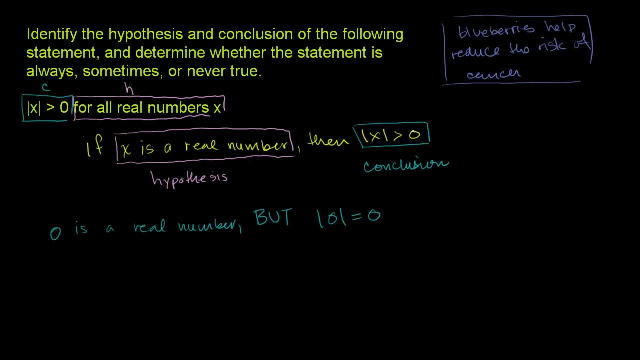 It's greater than 0. So this disproves this statement. It's definitely not always true. It's definitely not always true. Now, if you pretty much have any other real number, this will be true, Because any other real number is some distance away from 0..